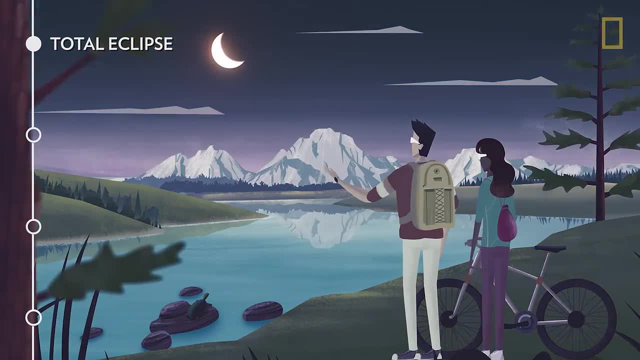 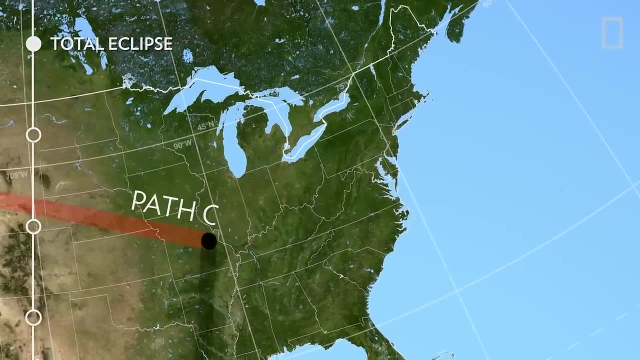 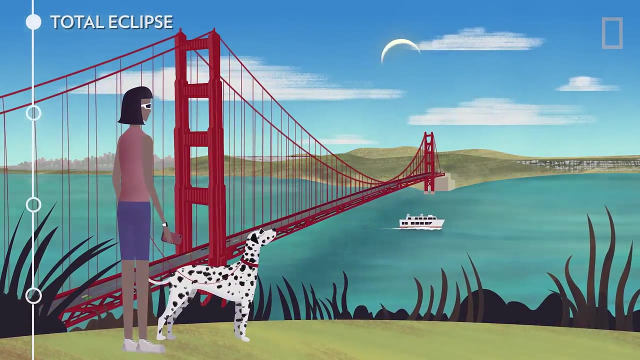 sun's surface. A total eclipse can only be seen if you're standing within the umbral shadow. That's why the imaginary line created by this shadow as it races across earth is known as the path of totality. People within the penumbra shadow see only a partial eclipse. 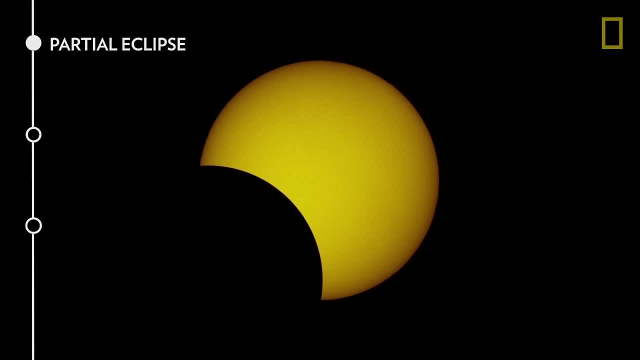 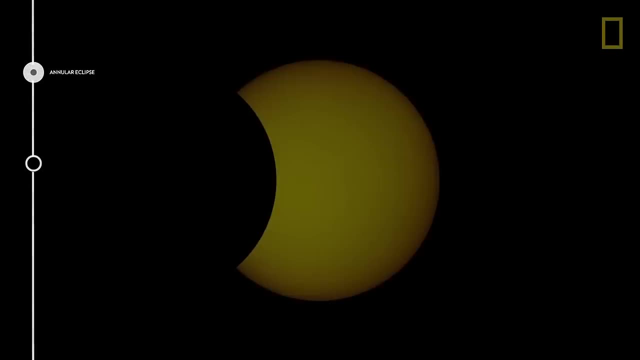 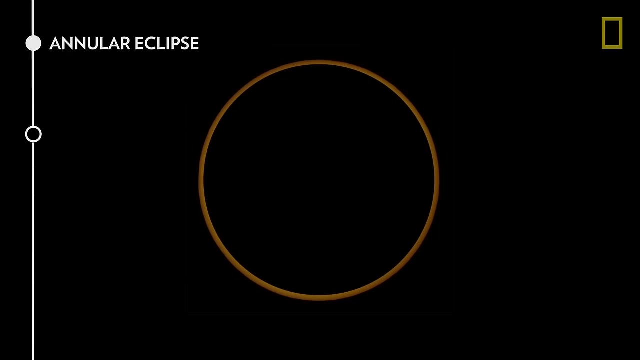 the second type. From this view, outside the path of totality, the moon passes in front of the sun, off-center, never fully covering its surface. Third, an annular eclipse occurs when the moon passes directly in front of the sun. However, unlike a total eclipse, the moon appears too small to fully cover the sun. 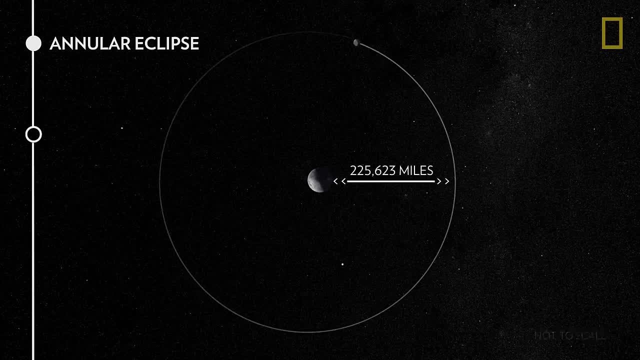 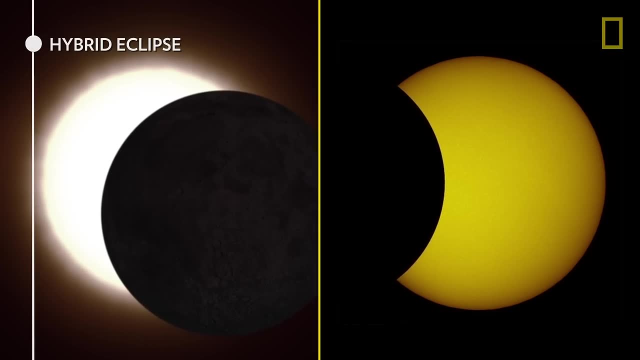 The moon's orbit is elliptical, so sometimes it's closer to earth and sometimes it's farther away. Last, a hybrid eclipse is when the moon's position between the earth and sun is lower. This happens when the moon passes in front of the sun off-center, never fully covering 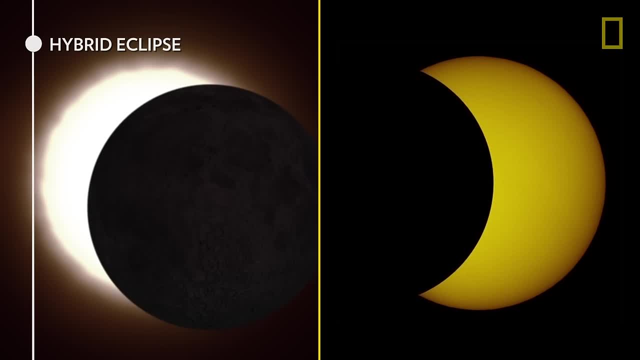 its surface. A total eclipse is when the moon passes directly in front of the sun and the moon's is so finely balanced that the curvature of the Earth plays a role. The Moon will be farther away from some parts of Earth along the eclipse's path. 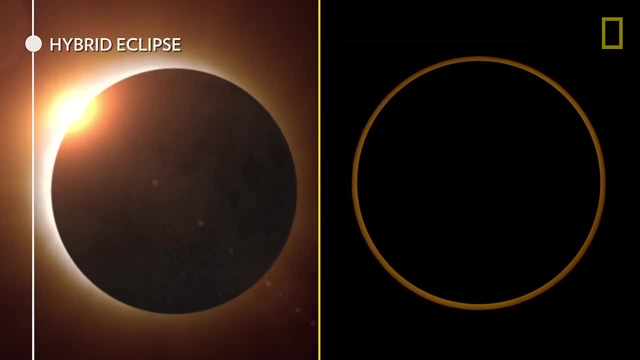 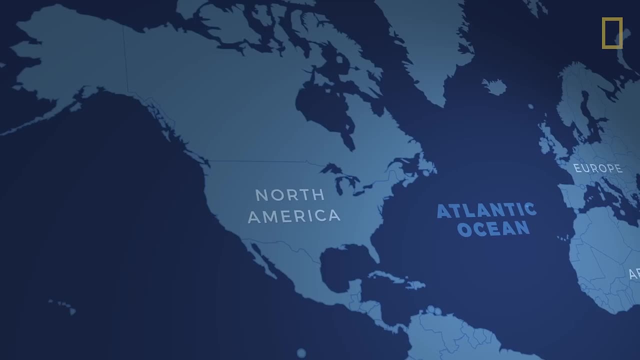 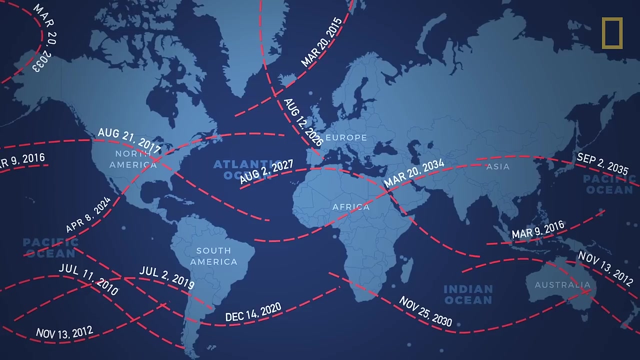 resulting in an annular eclipse. In other parts, the Moon will be just close enough to fully cover the Sun, resulting in a total eclipse. While a total solar eclipse happens somewhere on Earth every year or two, any given point on Earth experiences the event only about once every 400 years. 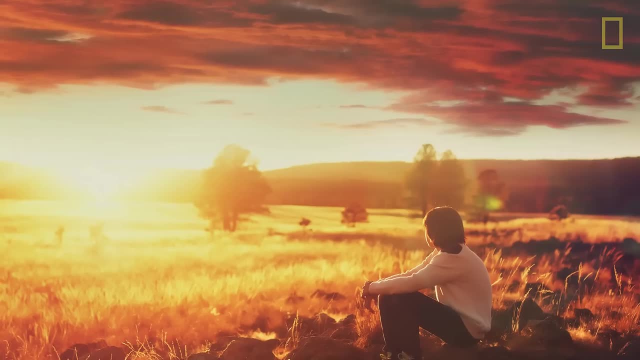 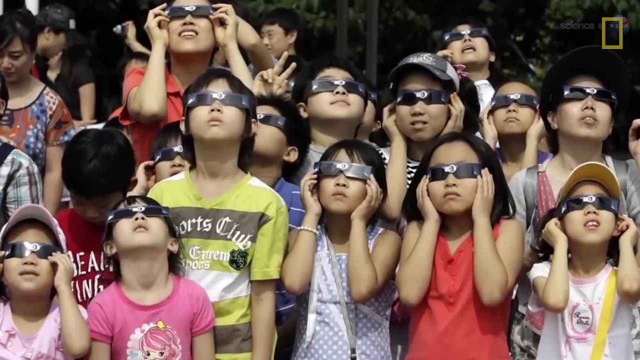 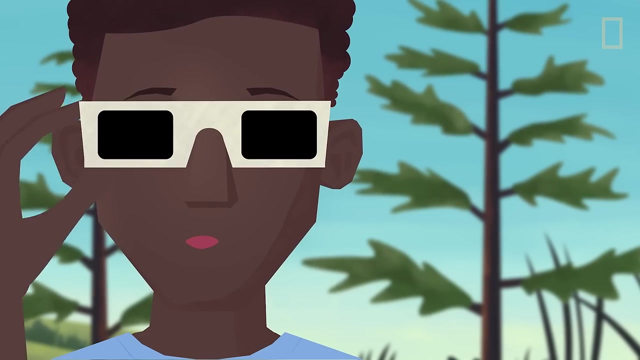 We interrupt this video for an important safety announcement. Looking directly at the Sun, even during an eclipse, can cause permanent eye damage. Fortunately, there are ways to enjoy an eclipse safely. The easiest is to use certified eclipse-watching glasses which are shaded thousands of times darker than typical sunglasses. 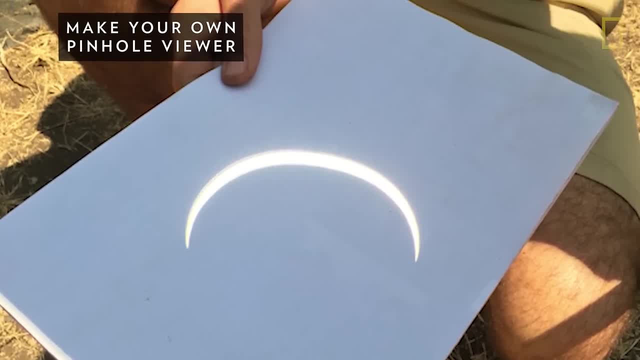 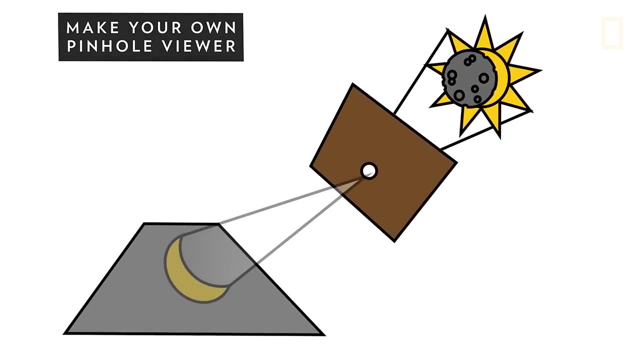 You can also look at the eclipse instantly and directly by making a pinhole viewer. Simply poke a small hole in a piece of cardboard, Hold the cardboard up to the Sun, allowing the Sun's image to be projected onto a flat surface. 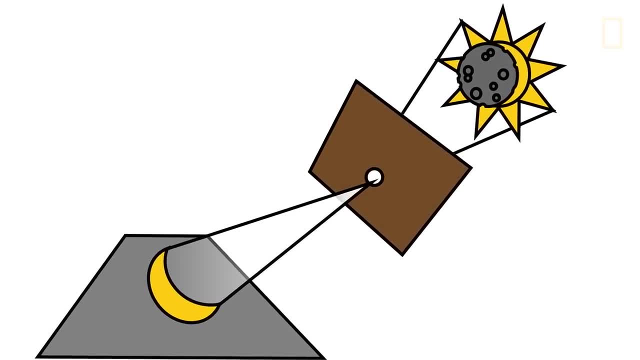 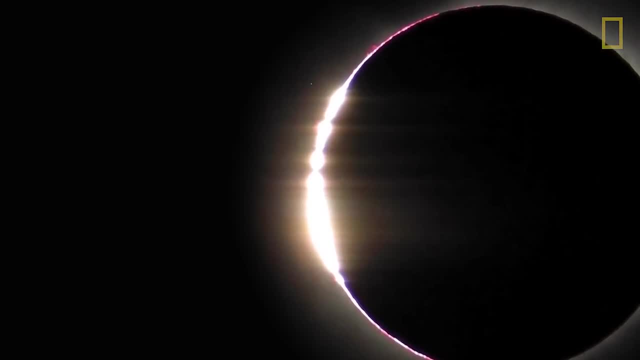 Be sure to look only at the surface and not through the cardboard. Just before the Moon completely covers the Sun, low-lying valleys on the Moon's edge will be the only spots that sunlight continues to pass through These remaining brilliant shafts of light known as Baily's beads.